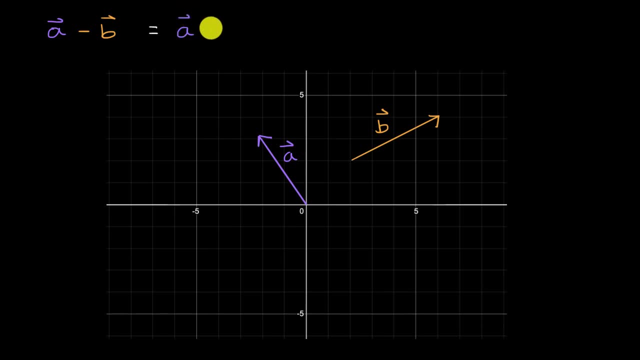 is the same thing as vector a plus the negative of vector b. Now, what is the negative of vector b look like? Well, that's going to be a vector that has the exact same magnitude as vector b, but just in the opposite direction. 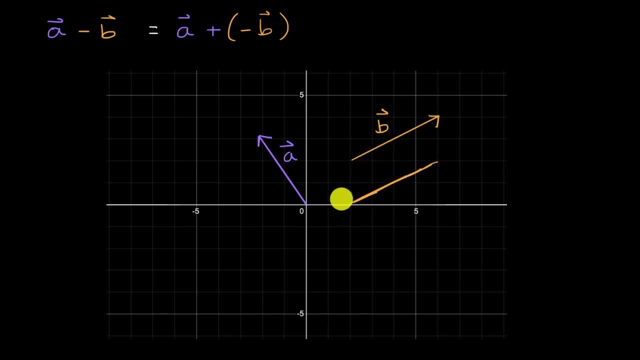 For example, this vector right over here would be the vector negative b. Now we just have to think about: what is vector a plus the vector b. What is the vector negative b? Well, there's two ways of thinking about that. I could put the tails of both of them. 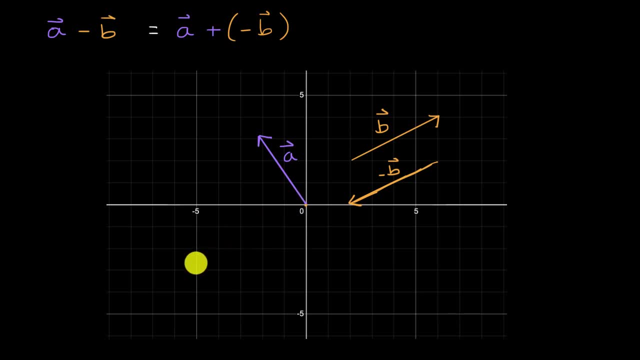 at the same starting point Might as well do the origin. So let me draw negative b over here, So we know the vector. negative b looks like that. So one way that you are probably familiar is you have vector a and then what you do is you take a copy. 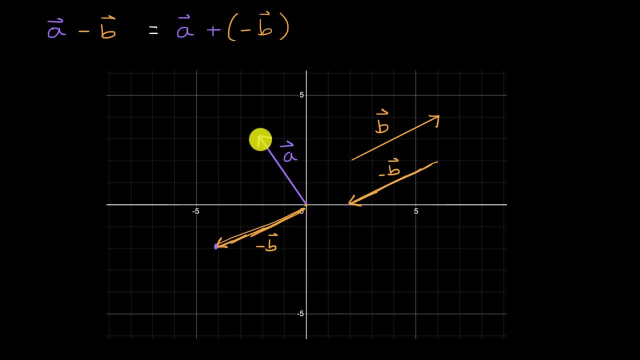 or you could think of shifting vector b So its tail starts at the head of vector a, And if you did that you would have vector a and then you would have vector b, And if you did that it would look like this: 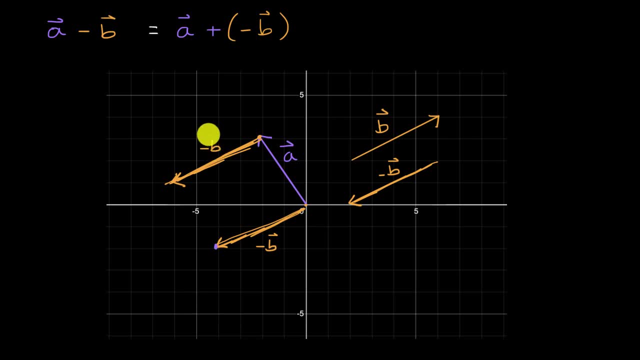 It would look like this: This is also the vector negative b, And then the sum of vector a and negative b. vector negative b is going to be going from the tail of vector a to the head of vector negative b, So this would be the result right over here. 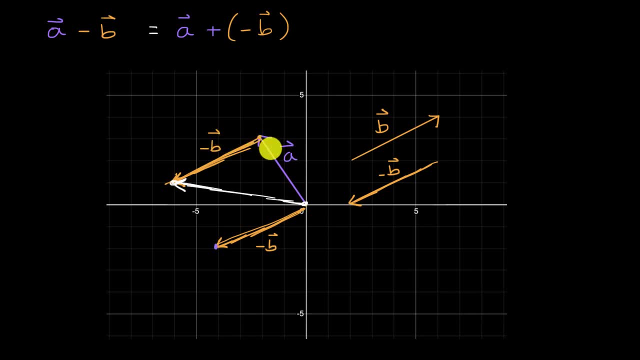 which you could view as the sum of a plus negative b, or the difference of vectors a and b, or vector a minus vector b. Now, if we want to think about it in terms of the parallelogram rule, we could take another copy of vector a. 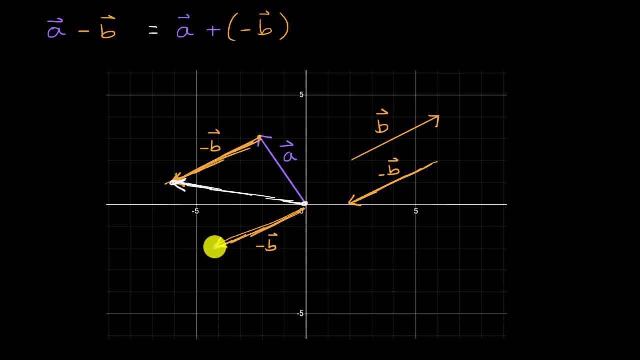 and put it so that its tail is at the head of this negative b, and then we would get it right over here and we are forming the parallelogram, And then the resulting vector is the diagonal of the parallelogram, And this just helps us appreciate. 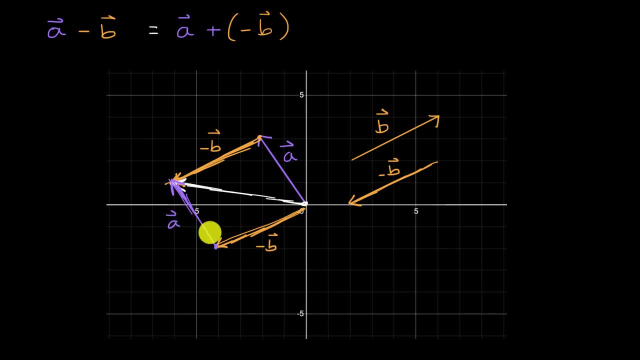 that we could start with negative b and then add vector a to that, or we could start with vector a and then add negative b to that. But either way, you get this white vector right over here, which we can view as the vector a minus vector b. And we're done.